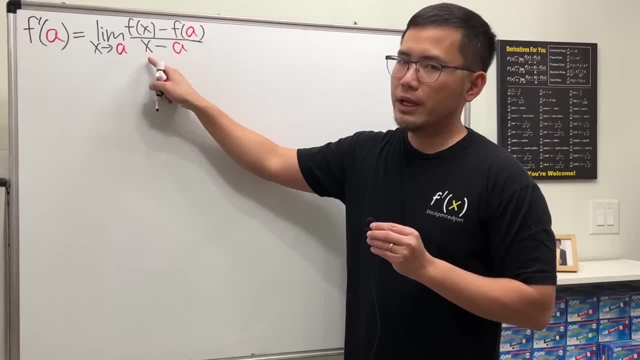 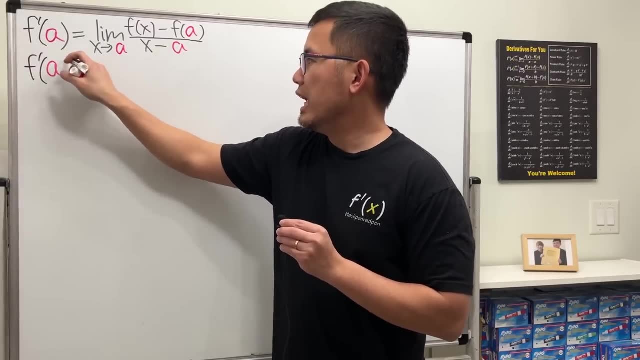 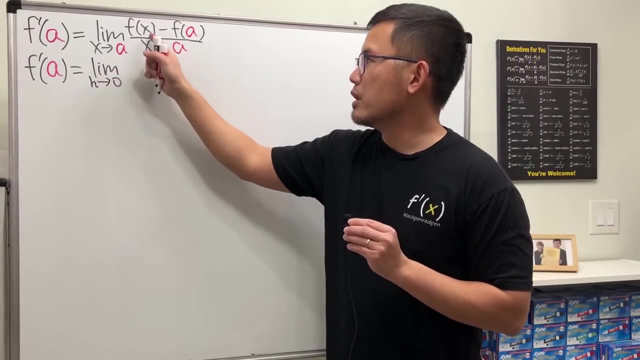 As you can see, we have y2 minus y1 over x2 minus x1.. Here is just the first version. The second version is the one with h. f' of a equals the limit as h approaching 0. And the h is the distance between this point and that point. 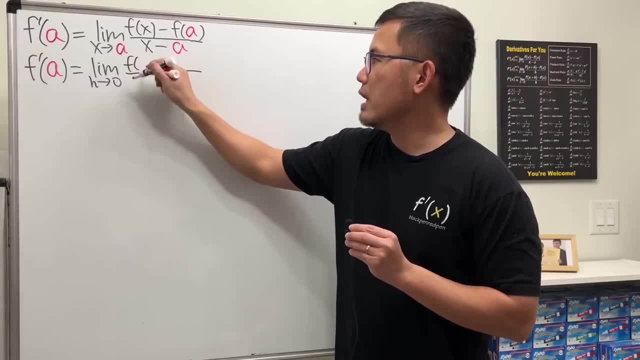 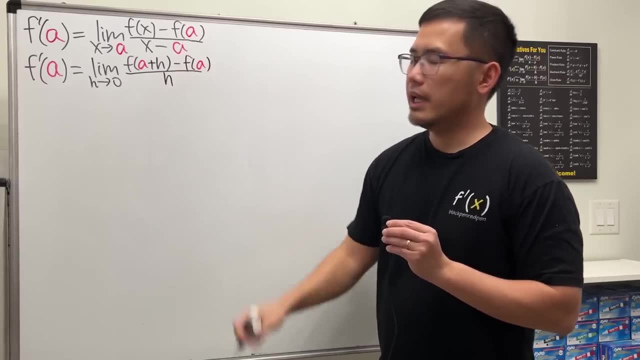 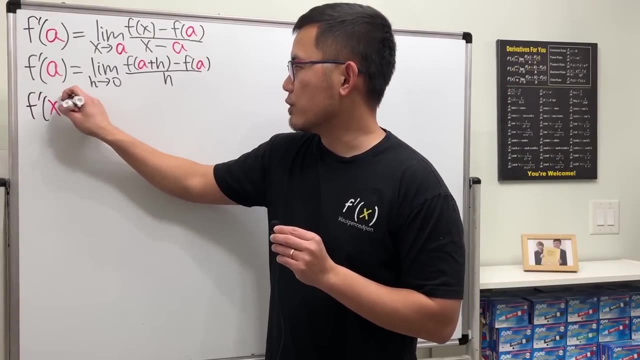 So what we will do is we will have f of a plus h, and then minus f of a, and then divided by just h. Why do we need a second one, though? Because of the following: This is the official definition of the derivative as a function. 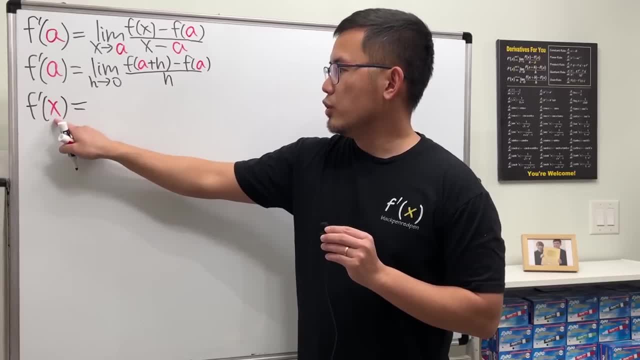 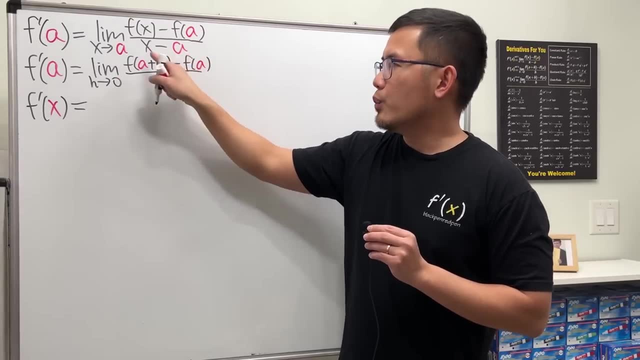 Here we have f' of x. Imagine if we put x into this a, That's okay. but if you put x into this a, that a and that a, Well, we get x minus x. No, you get 0 on the bottom. 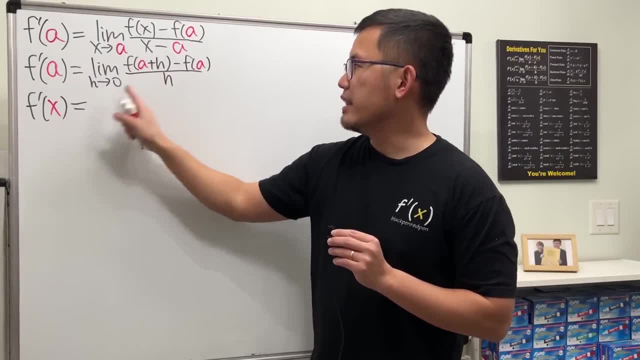 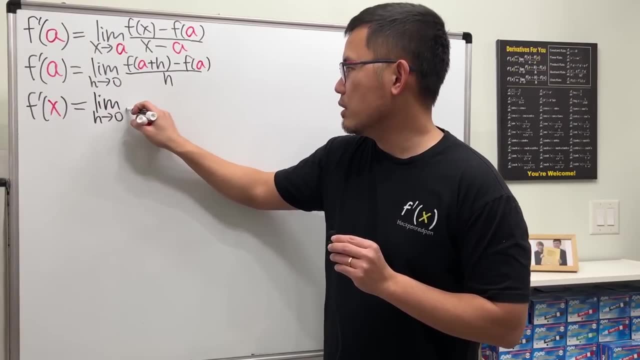 No good, But if you put x into this a, this a and that a, it's all okay. So that's why we need to use that. And this is the limit, as h approaching 0, of just replace all the a's with x's. 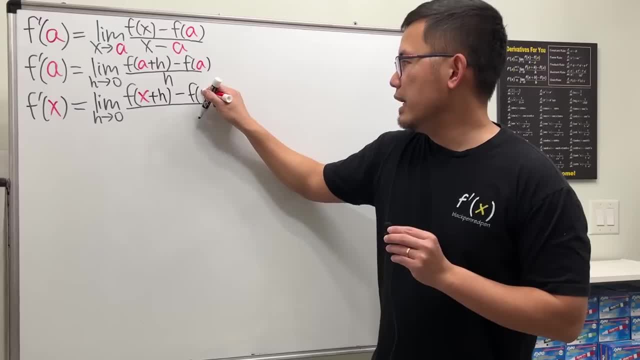 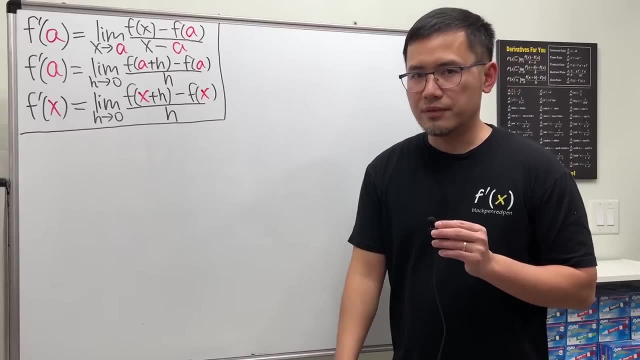 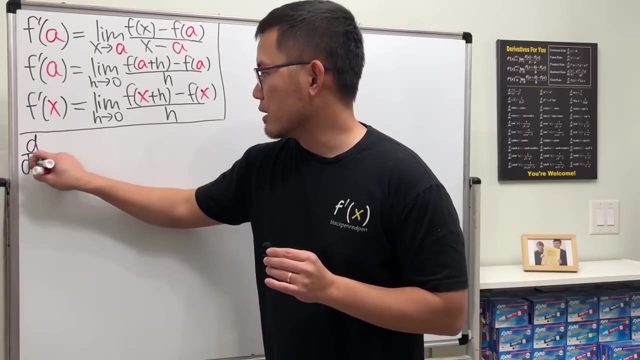 So x plus h minus f of x, And then all divided by h. And these are the definitions in terms of a limit for the derivative. After the definition, Of course, here are the differentiation rules. The first one: I'll put down the constant rule for you. 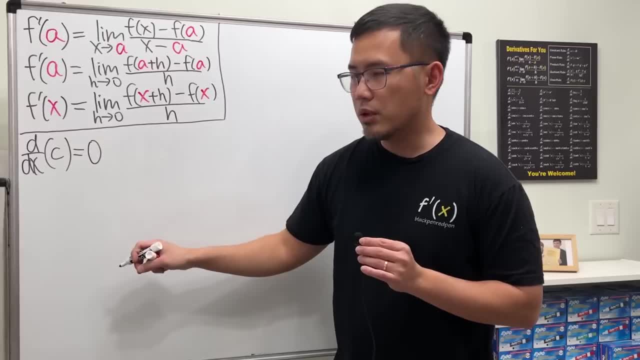 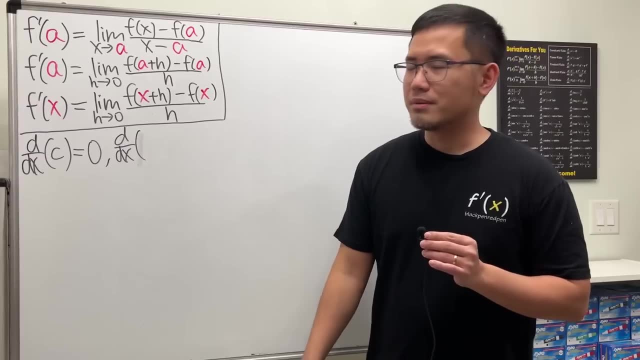 Taking the derivative of a constant c, it's just equal to 0.. And then the next one, everybody's favorite: Taking the derivative of a power function, x to some power that say n. Keep in mind x is in the base. 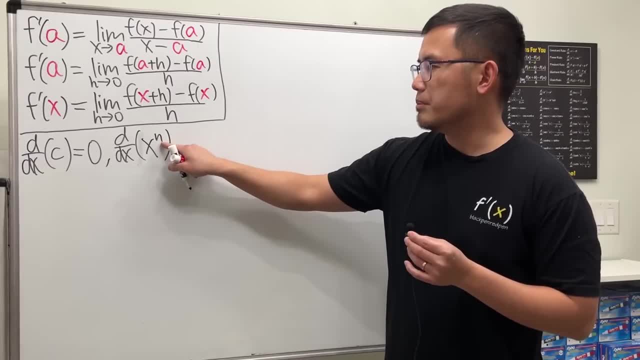 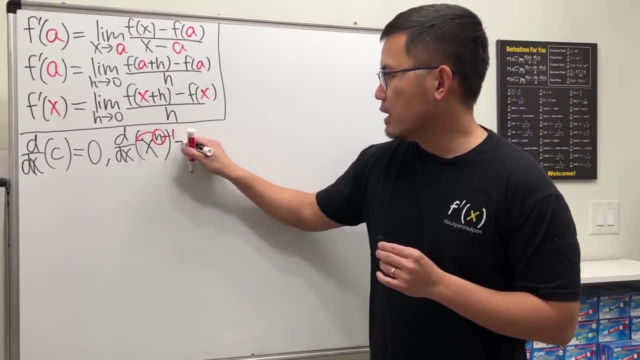 The n right here can be any number. It can be 17,, it can be pi, it can be negative 2, etc. For this situation, just put the power to the front and then minus 1, and we get n times x to the n minus 1 power. 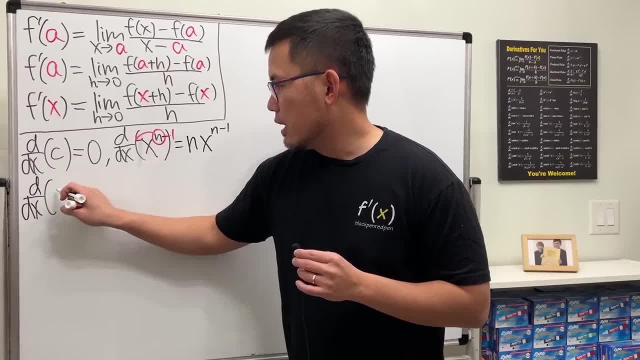 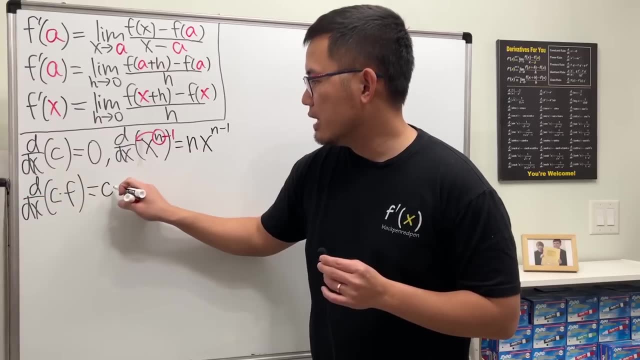 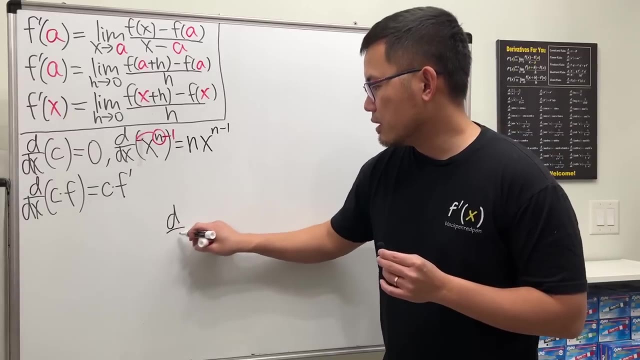 Now let's say, if we have a constant multiple with a function, So c times f, For this one you can put the c on the outside and then just multiply by the derivative of f, So f prime, like that. So just a real quick example: if you're taking a derivative of, let's say, 3x to the fifth power, 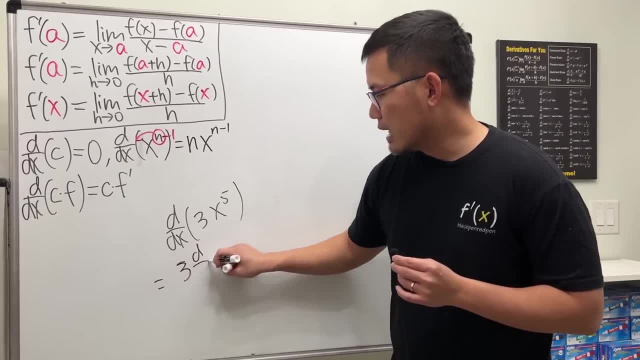 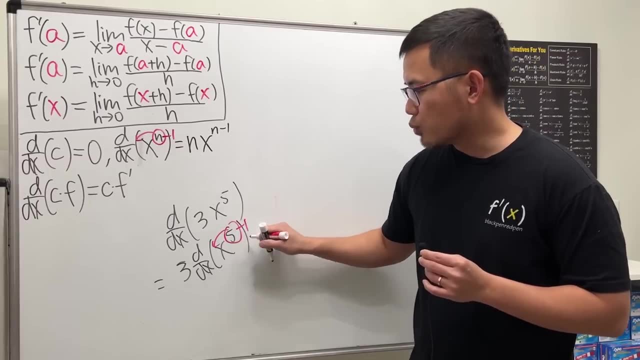 Well, you can put the 3 on the outside and then focus on taking the derivative of x to the fifth power. To do this, use the power rule. Put the power to the front minus 1. So you have 3 times. this is 5x to the fourth power. 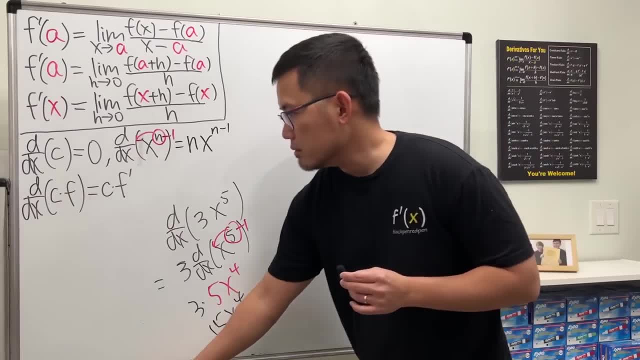 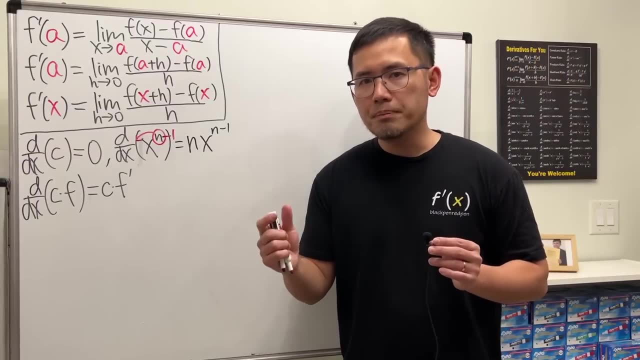 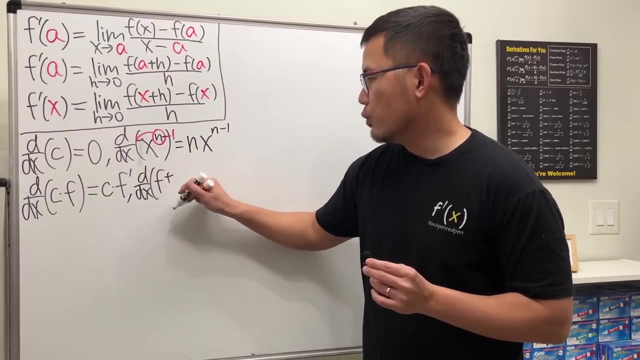 And then just multiply, get 15x to the fourth. So that's what that is for. And then the next one is if we're taking the derivative of a sum or a difference of two functions. So d, dx, let's say we have f plus or maybe minus g. 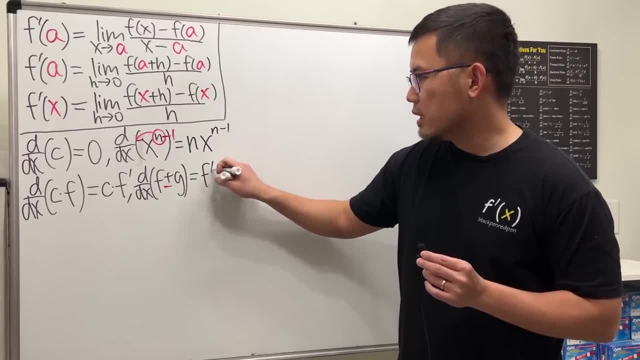 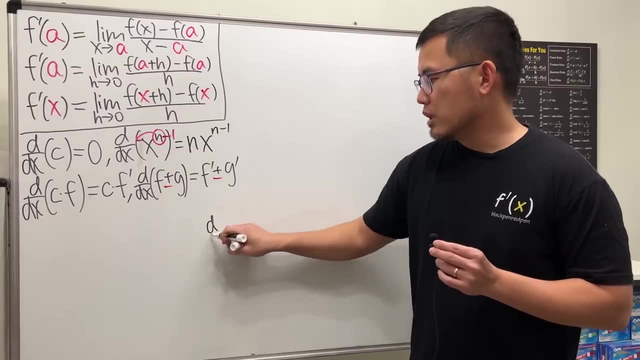 For this you can just go ahead and take the derivative of the first one and then add it with the derivative of the second one, But if it's a subtraction you just subtract instead. So if you are taking a derivative of x squared plus x to the third power, 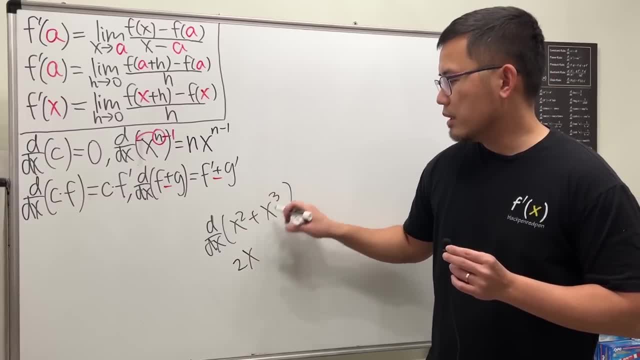 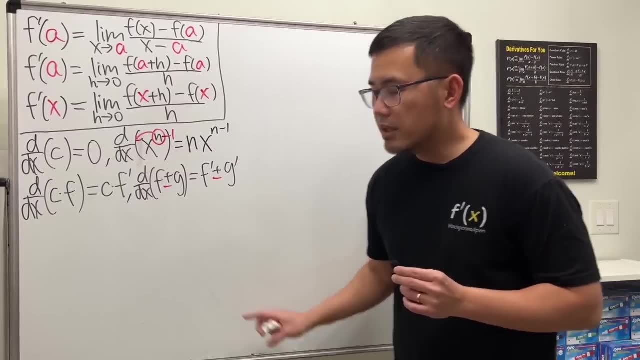 just do the power rule here You get 2x to the first power And then you do the power rule right here and add them up 3x squared. So that's that After the sum or difference. of course we can also talk about the product rule. 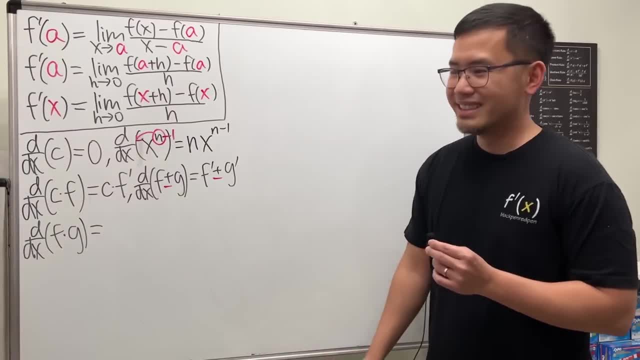 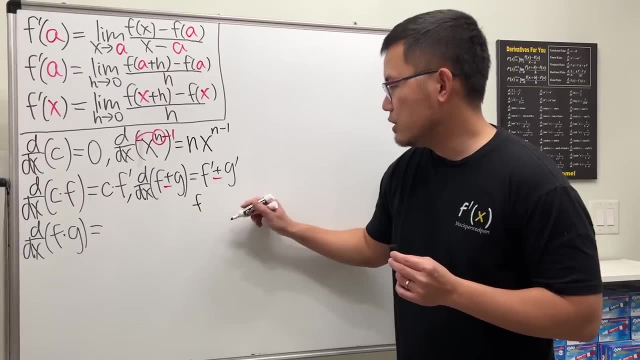 And this right here, it requires you to remember it. Right here I will have a way for you guys. Let's write down the f first right here, and also the g right here, And then we are going to just differentiate them separately. 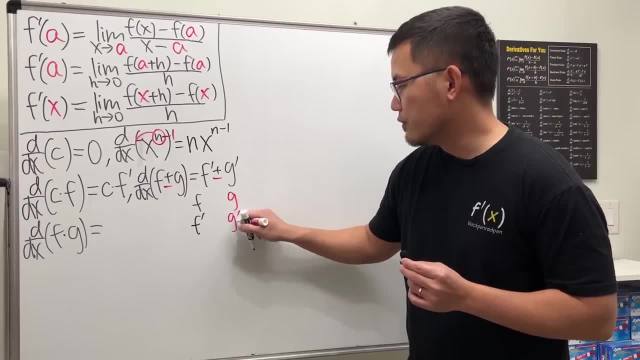 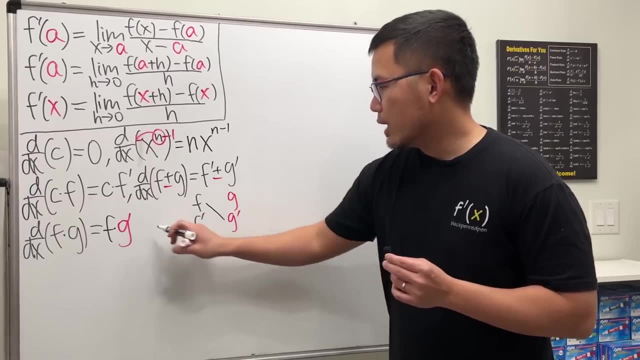 The first function, differentiate that, And then the second function, differentiate that, And then you do this: times this, Which we get f times g prime. And then we are going to add this with this: times that Which is g times f prime. 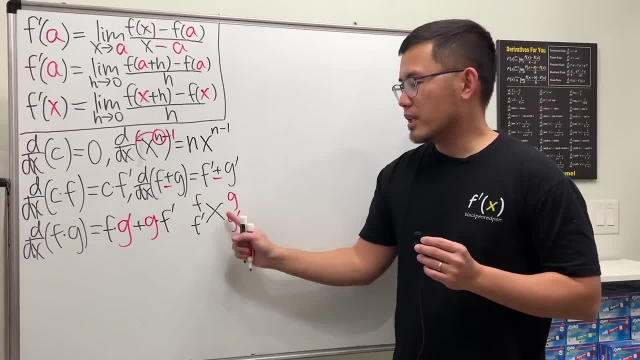 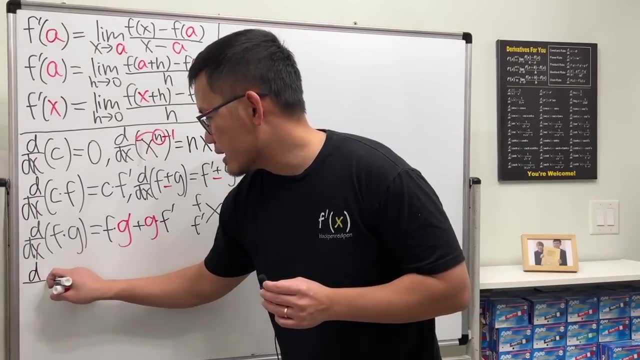 Especially if you are doing derivative for the first time. this right here will be really, really helpful. You can check out my other videos for worked out examples for that. After the product, of course, we have the quotient, So we have f over g. 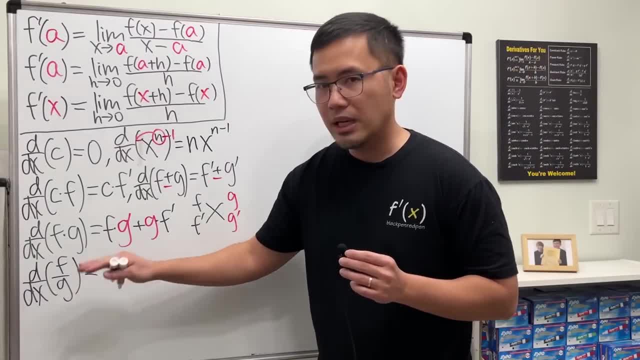 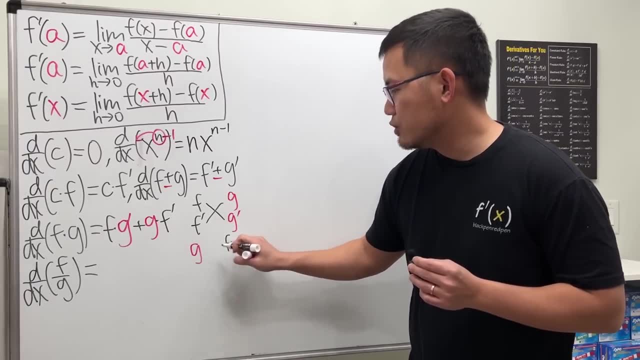 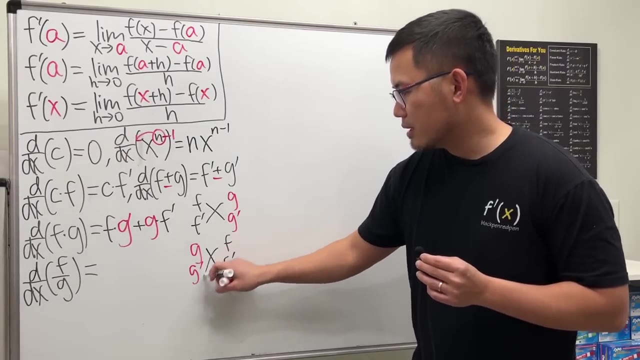 For this one, remember- quotient is stable, So we have the opposite of a product. Instead of putting down f and g, let's write down g and f. g goes first, And then just differentiate this and differentiate that. Let's still do the same thing. 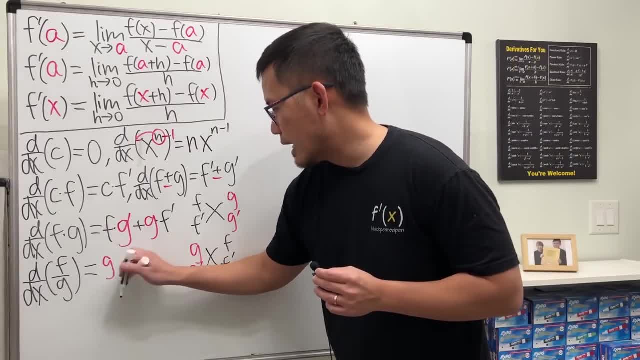 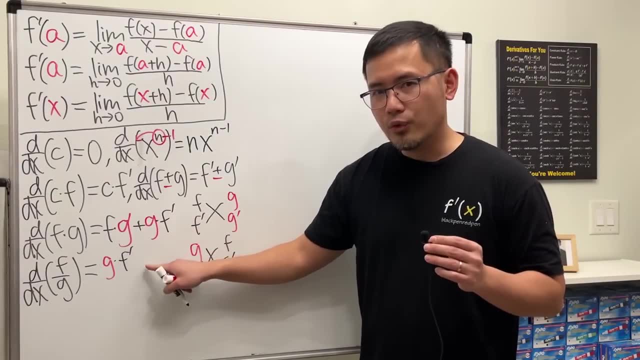 g times f prime. That will go to the top. And then remember, it's the opposite: For product rule we add, For quotient rule we subtract, And then we just do this times that f times g prime, f times g prime. 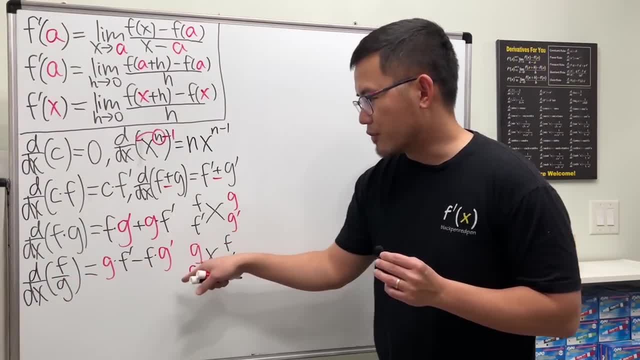 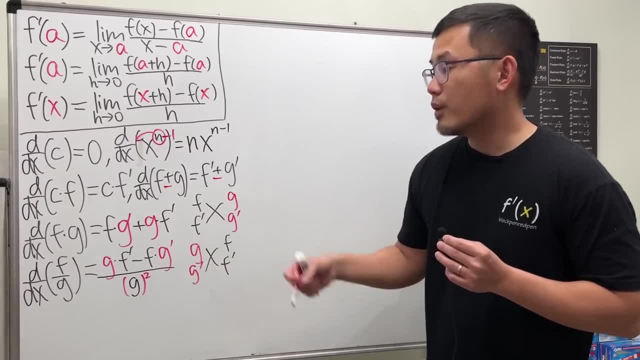 And if we started with a fraction, we'll end up with a fraction as well. We are going to divide this by the denominator g to the second power. Why is this true? You can check out my other video for it, The next one, of course. 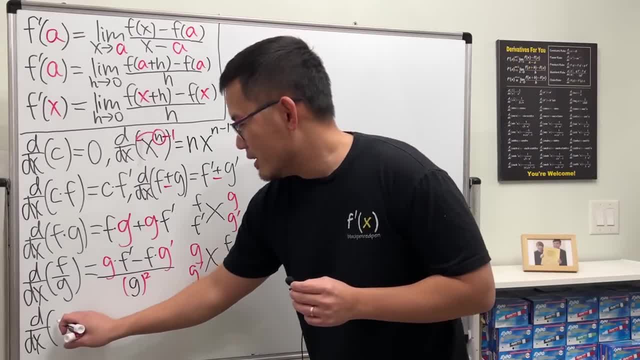 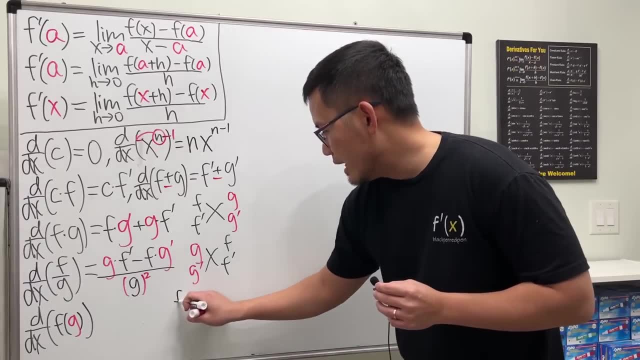 everybody's least favorite, The chain rule. It's a composition of two functions, That's the f of g. This is how you can do it. You have f of a box, f of something. Inside of the box is the g function. 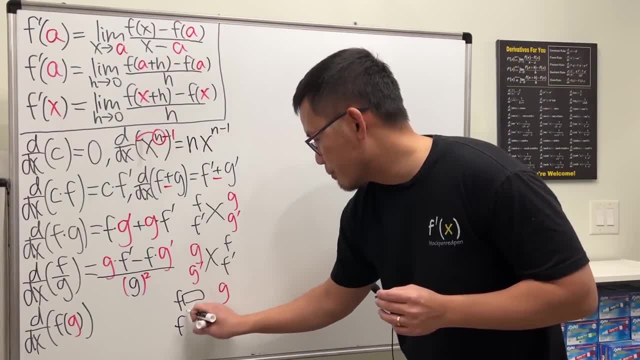 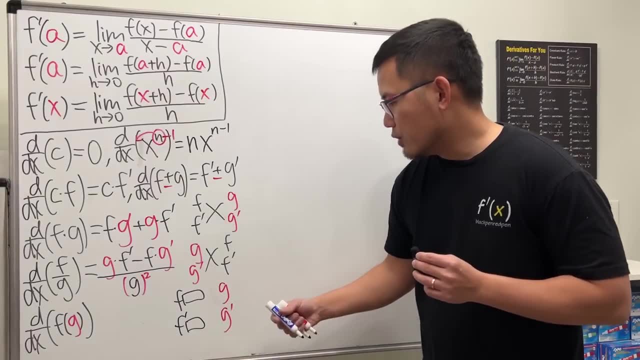 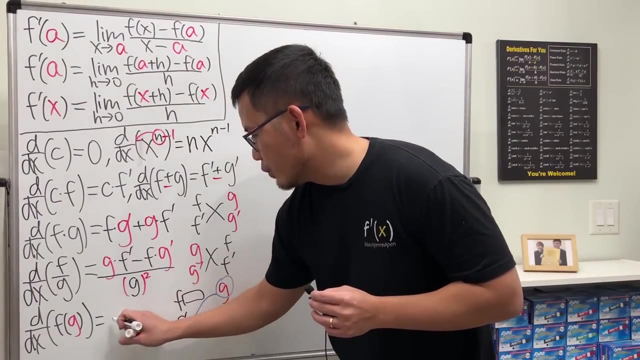 Take a look at this and take the derivative f prime of a box. And then take a look at this and take the derivative g prime For this. just go ahead, put the g function back to the box and then multiply. So right here in the math notation. 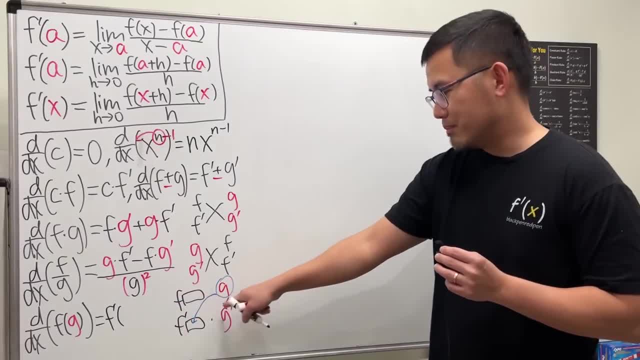 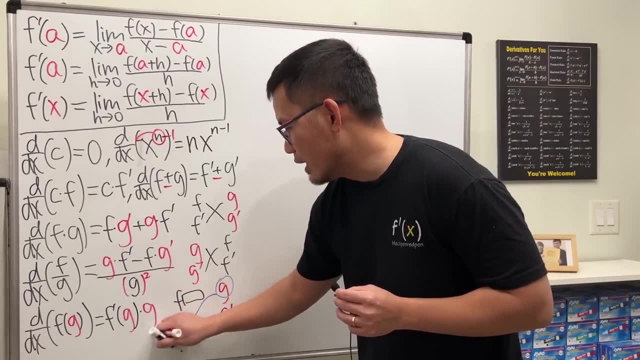 we get f prime. Use parentheses for the formula, But the box will help you to understand. Inside you still have the g function. It stays the same, But on the outside you have g prime that you have to multiply. That is the chain rule. 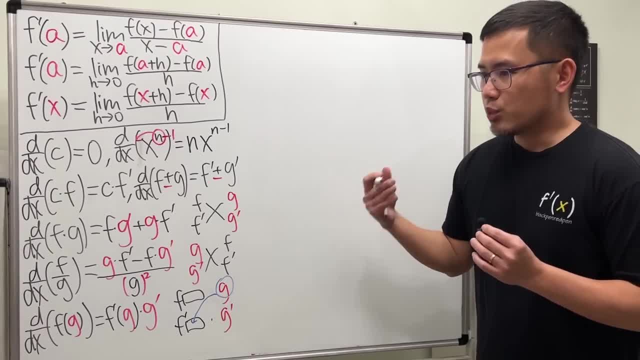 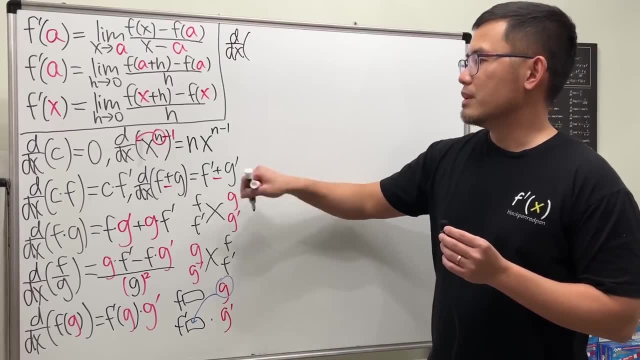 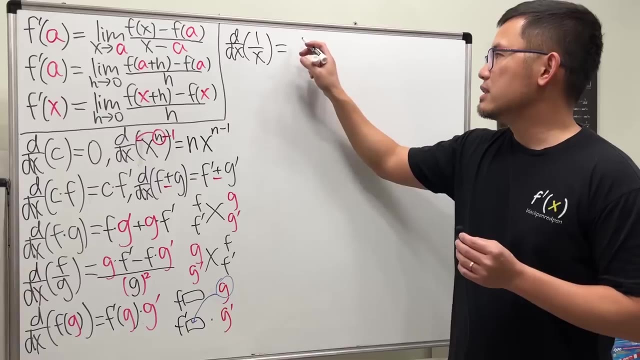 So these are all the differentiation rules. Now here are the derivatives of the usual functions that you have to know. Let's start with the derivative of some situation from here: 1 over x. This is a very common one, I think you should remember. 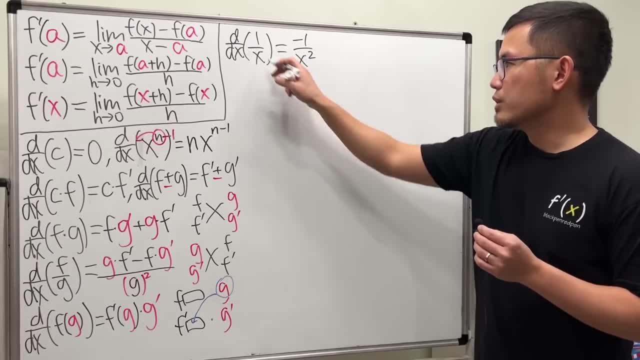 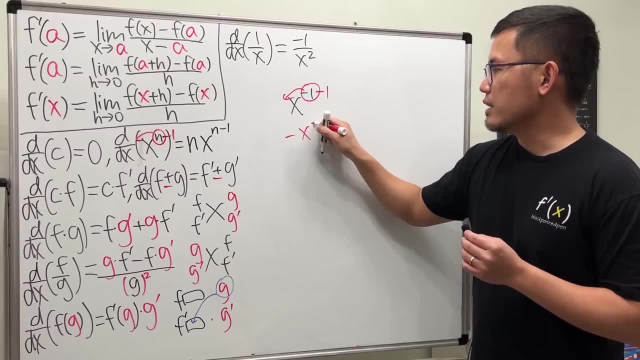 For this right here. the reason is: just look at this as x to the negative 1, and then bring the power to the front, minus 1. We get negative x to the negative 2.. That's how we do it, But it will happen quite often. 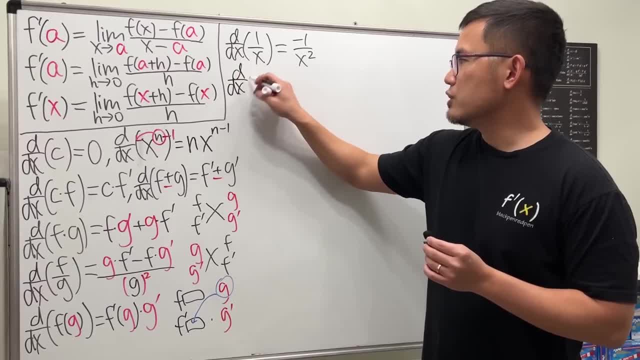 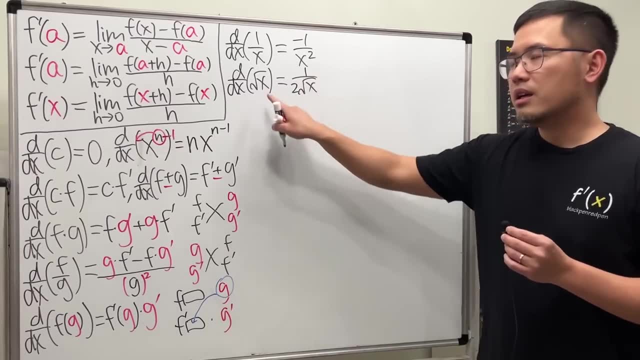 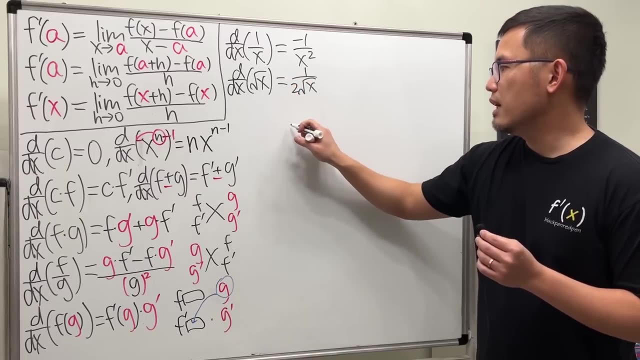 It's easier if you remember it. Another similar situation is you differentiate square root. If you remember this, you get 1 over 2 square root of x. You will be dealing with square root functions a lot. You should remember it. Why is this true? 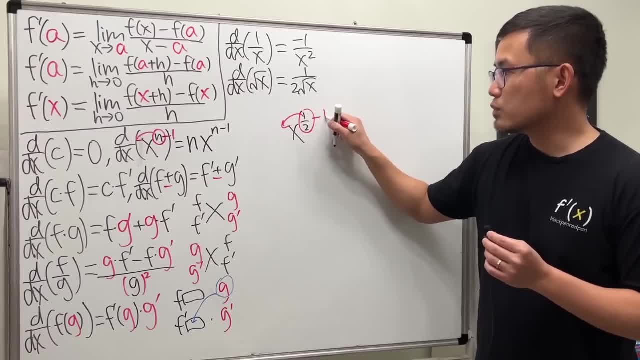 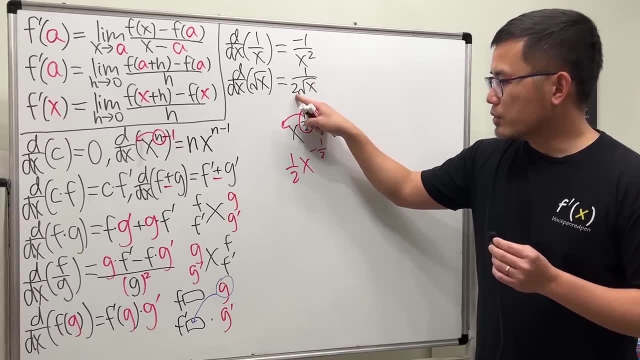 Because look at this as x to the 1 half power, Put the power to the front minus 1. We get 1 half, x to the negative 1 half. So you see we have the 1 over 2 and x to the negative 1 half. 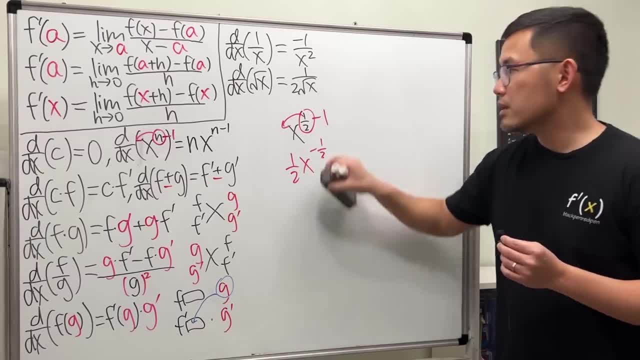 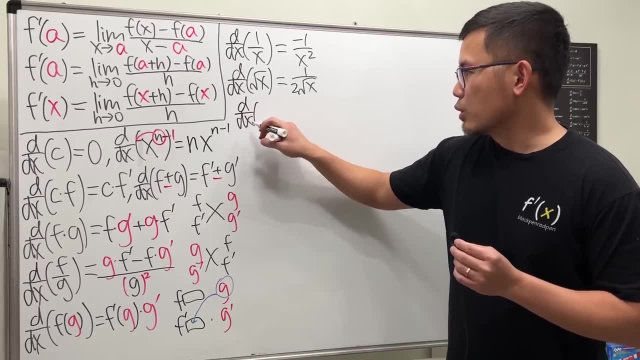 goes to the bottom. 1 half power is the square root. Now let's talk about exponential functions. The first one, of course, the derivative of e to the x. This, right here, is very beautiful. It's still just e to the x. 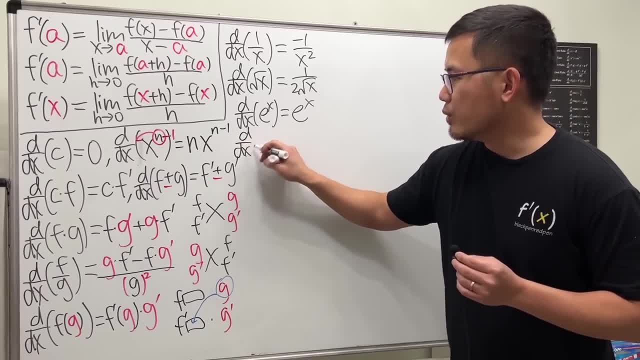 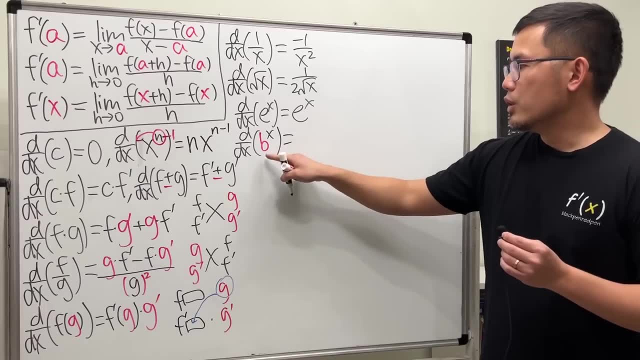 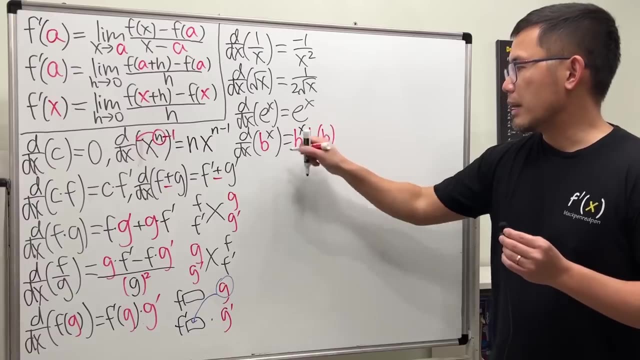 But if you are talking about the general case, when you take the derivative of, let's say, a base b to a power x, this right here you first repeat it: You have b to the x power, but you multiply by natural log of that base b. 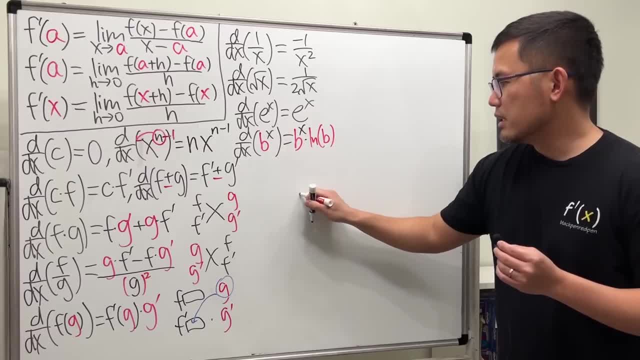 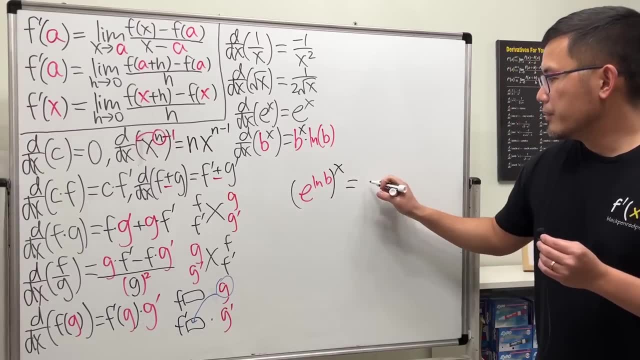 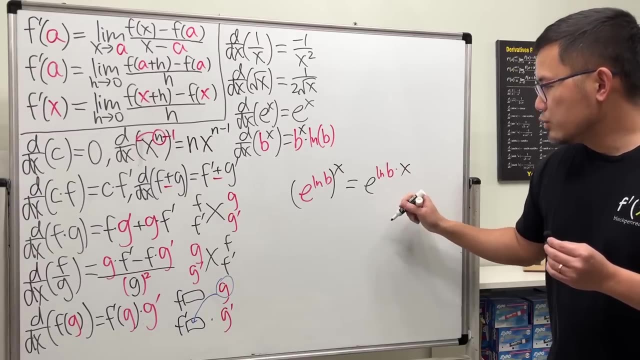 The reason why is because we can look at this b as e to the ln b power and then raised to the x power, so the function is just e to this times that. so we have ln b times x power, Taking the derivative of this, this thing right here. 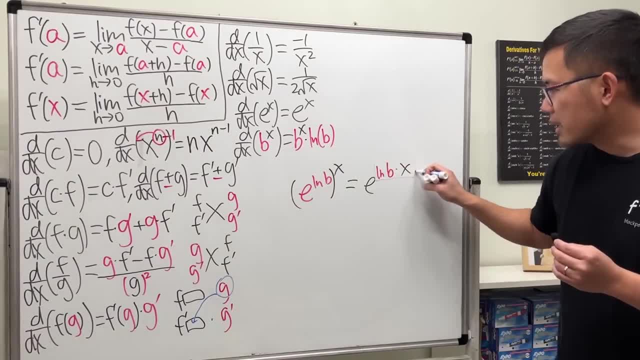 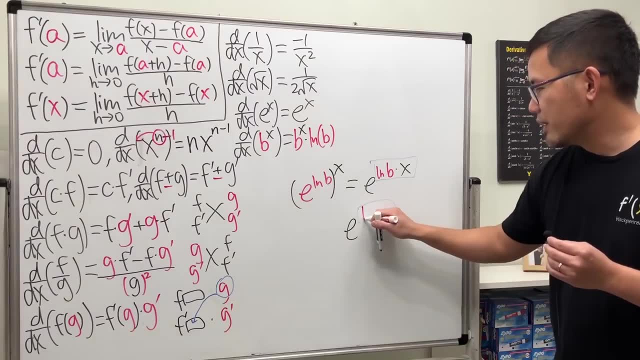 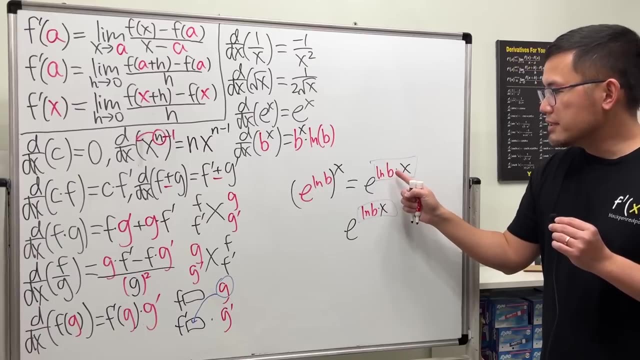 repeats first because it's like e to a box, So the box e to the same box, it stays. And then you have ln b times x, But look at the box and then differentiate that This right here is just a number, so a number times. 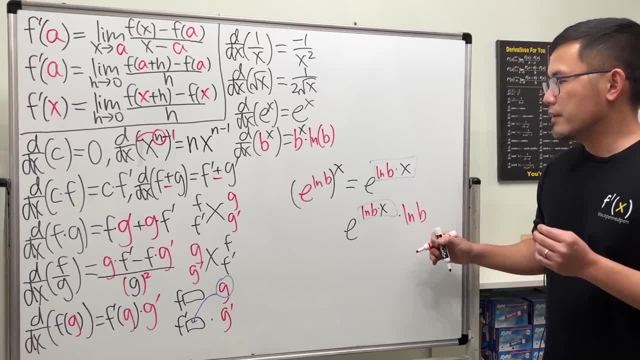 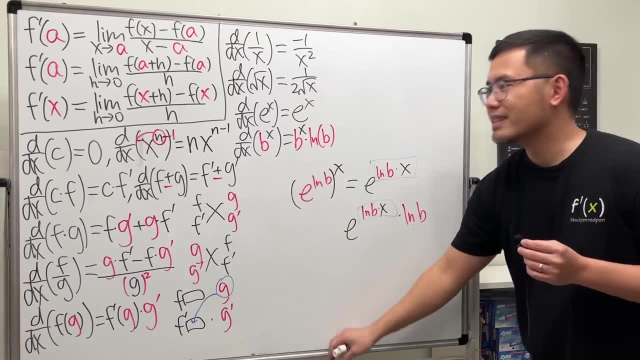 x, the derivative is just that number: ln b. So that's why we have the ln b, and this right here is just that, which is just that which is just b to the x. So that's the general case for the exponential function. 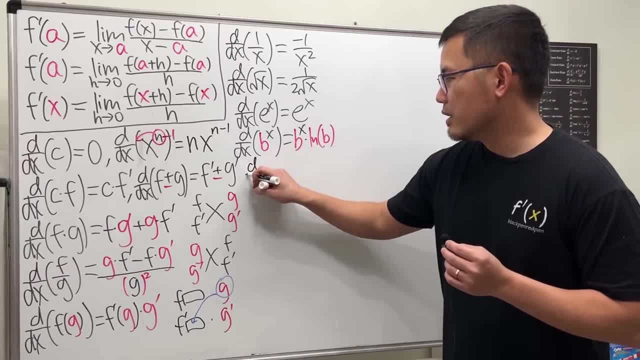 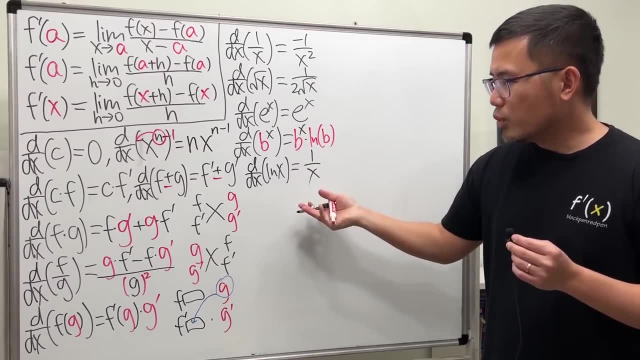 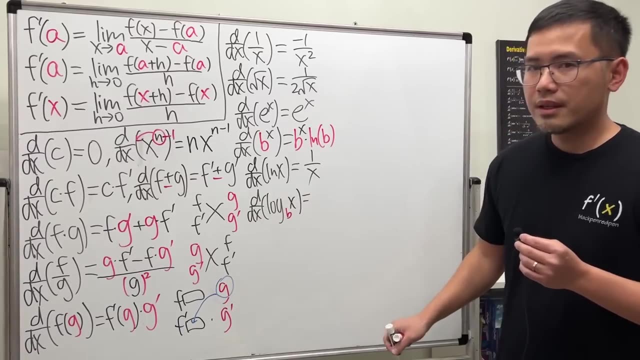 Now the inverse of them, of course. here is the derivative of natural log. Here we get 1 over x. But the general case for that is taking the derivative of log base, b times ln, x. This right here is similar to this. 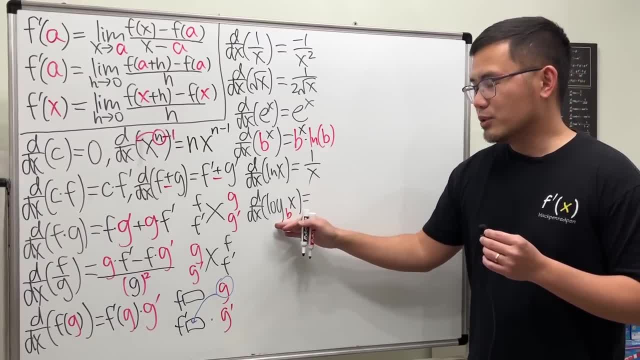 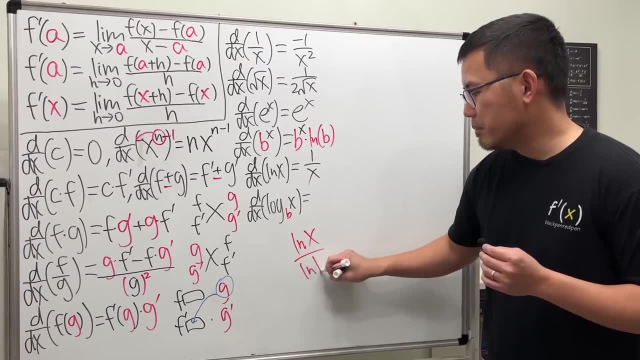 and same idea. right, similar idea to this. Or you can just use the change of base formula for this. It's easier that way. actually, This is the same as saying ln x over ln b. right, take the derivative of that. 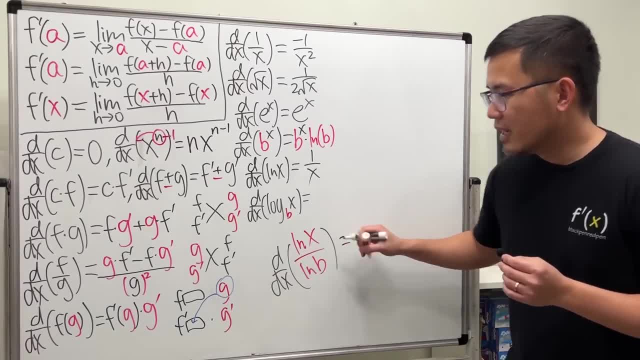 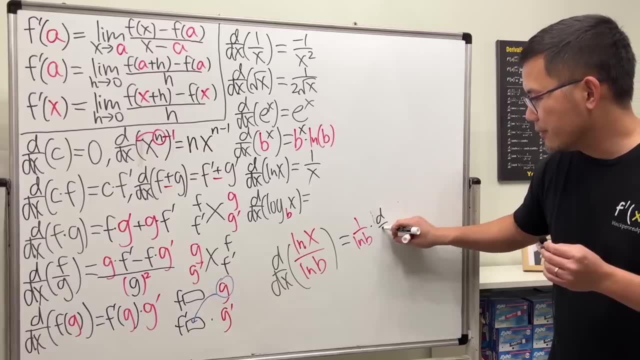 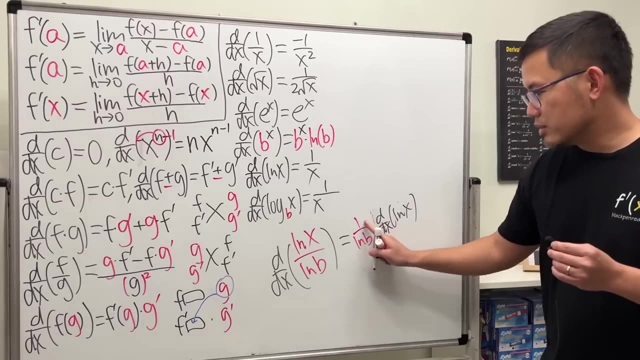 And we can put the 1 over ln b to the front by this rule. So we have 1 over ln b times the derivative of ln x. What's this? That's precisely 1 over x. And remember, this is just a constant. 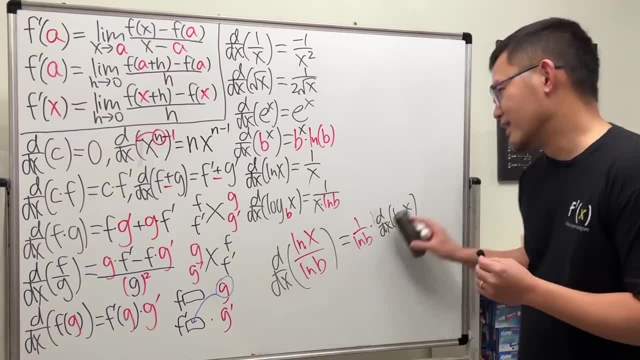 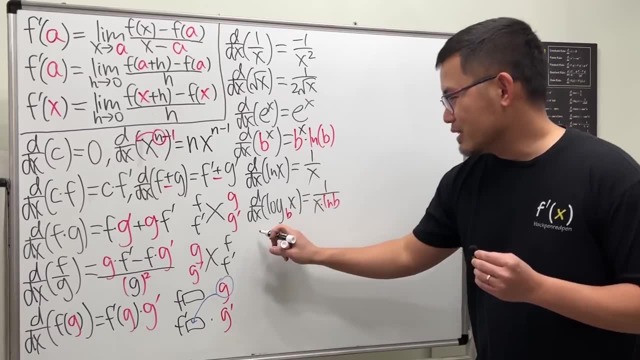 so let's multiply by ln b on the bottom. So that's how you get that. Now, these are all the non-trick functions, and you know what's coming. The next one: let's put down the derivative of sin x, And let's also put down: 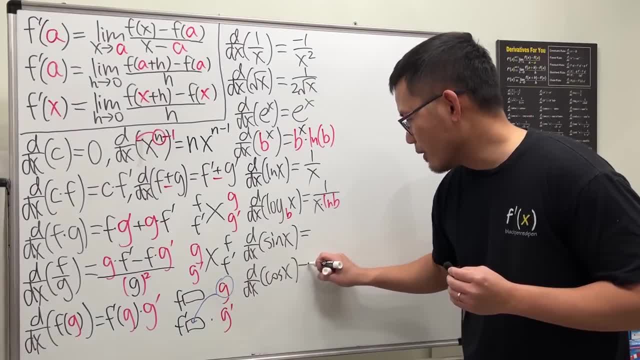 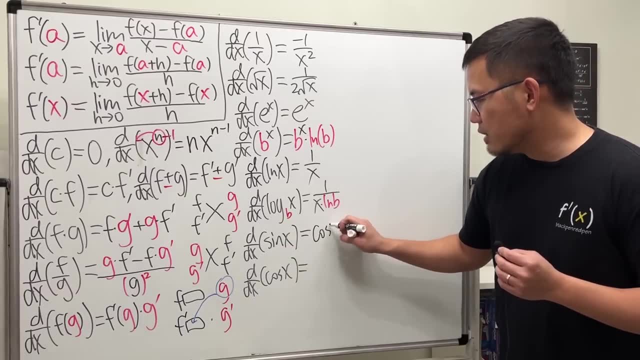 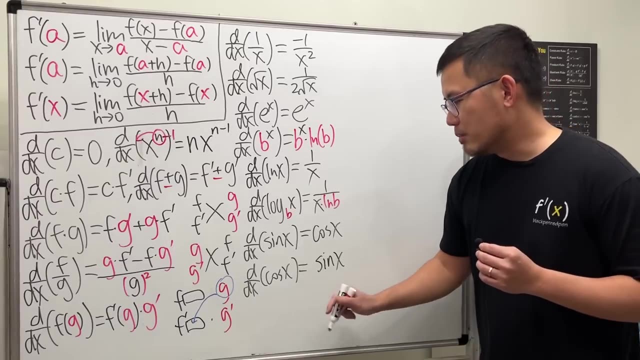 the derivative of cos x right here as well, Because sin and cos, they are best friends in calculus. The derivative of sin x is positive cos x. The derivative of cos x is sin x. But one way to remember that this is negative, because 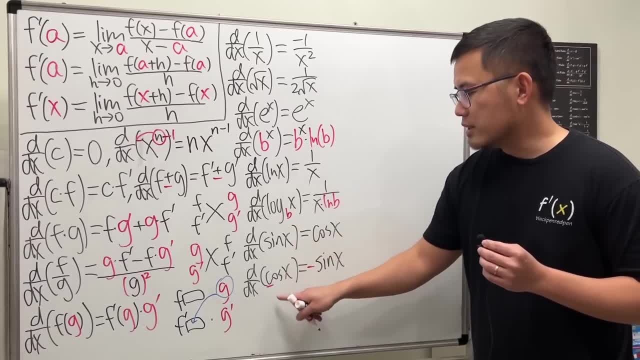 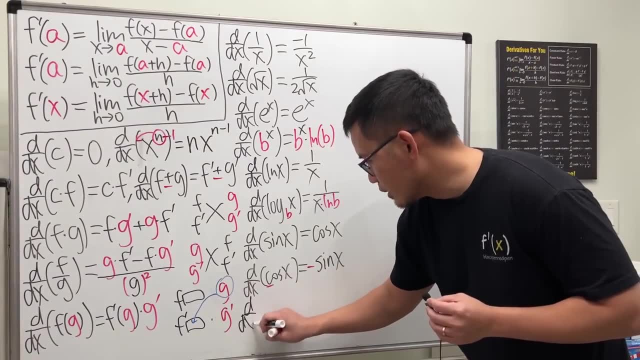 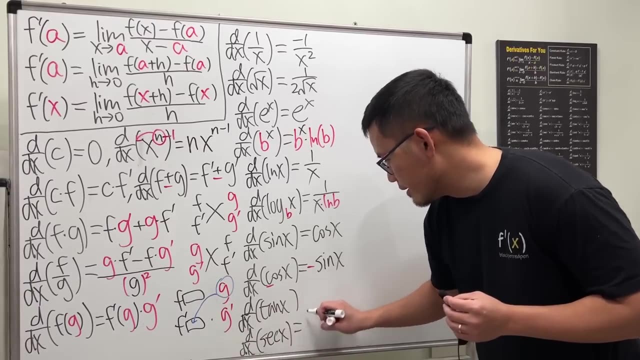 cos starts with a c, All the trick functions that start with a c, you have negative derivative, so negative sin x for that. Next let's take a look at the derivative of tan x and also the derivative of sec x. They are also best friends. 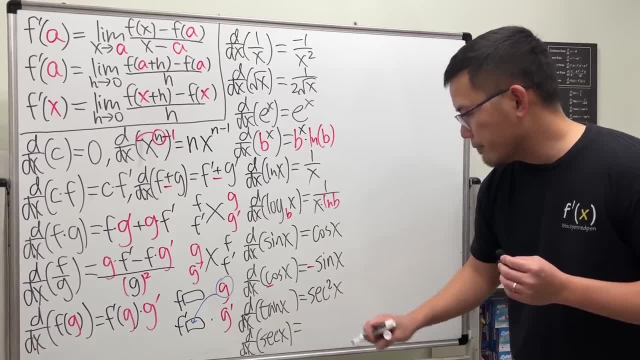 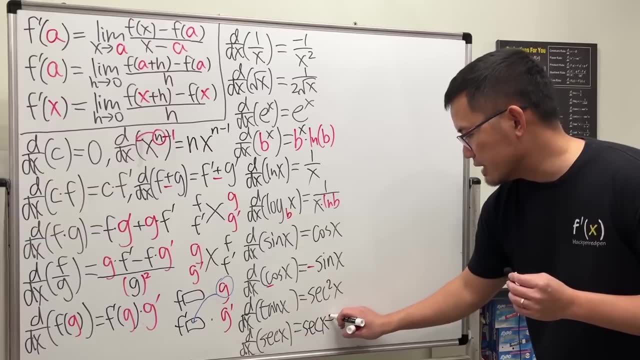 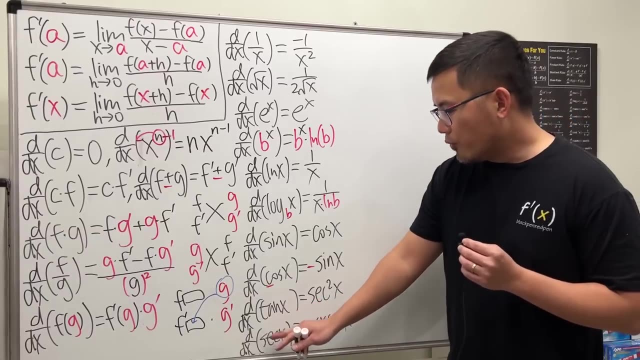 The derivative of tan x is sec x. The derivative of sec, it first repeats: you have sec x and then invites best friend, which is tan x. They are both positive because you don't have c. Now, if you are looking at the co-functions of, 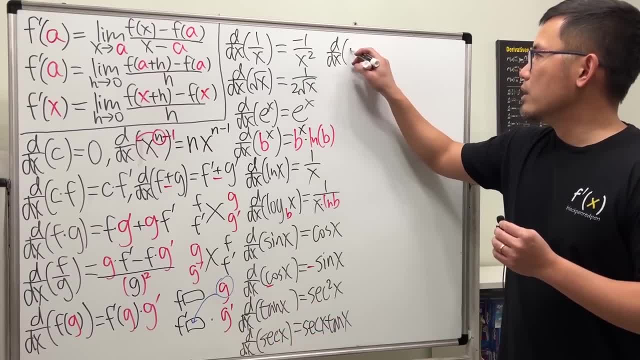 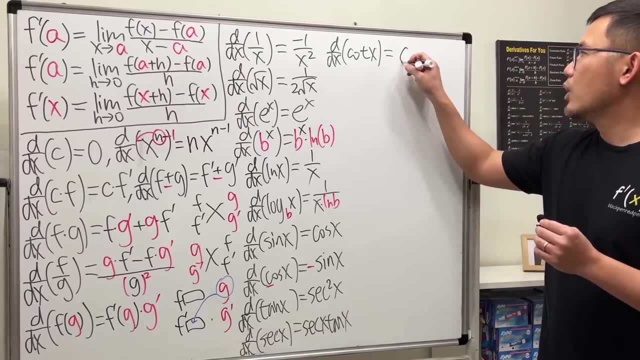 this and that. if you take a look at the derivative of the co-function of tan, of course cot x- well, it's the co-function of this. you get cos, sec x, But you see the c, so you have negative derivative. 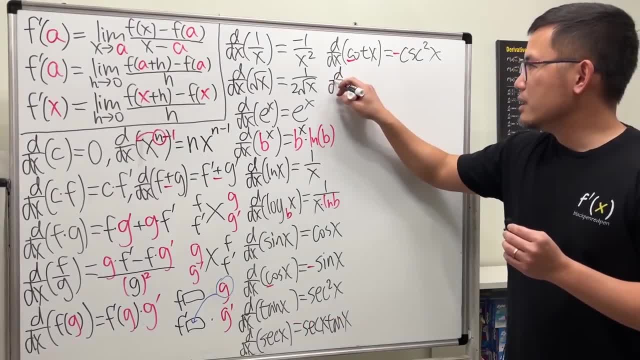 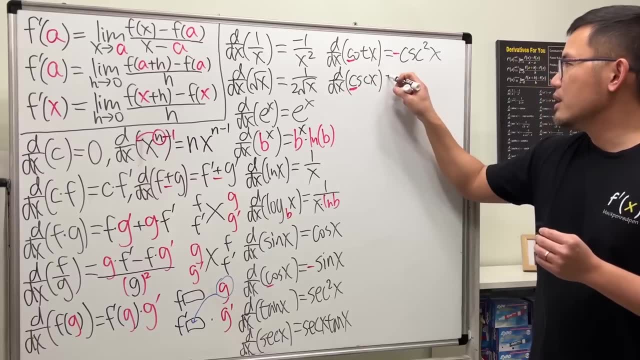 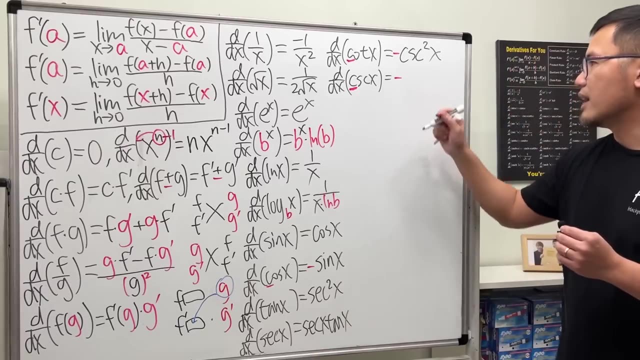 Likewise, when you have the derivative of the co-function of that which is cos, sec x, you know right away the c. you should get negative derivative: Same thing, It repeats, right, And then just a co-version of that It repeats. so you have the. 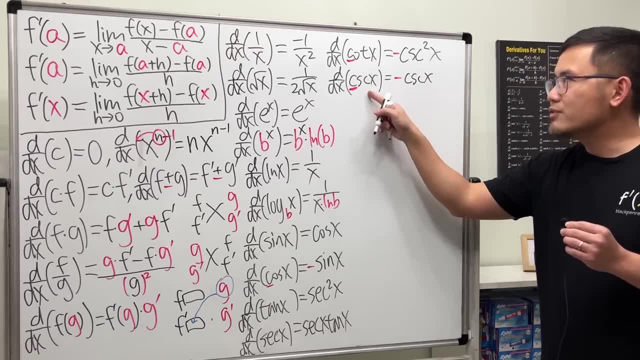 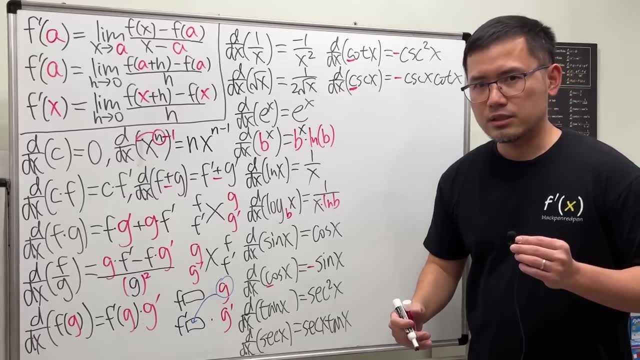 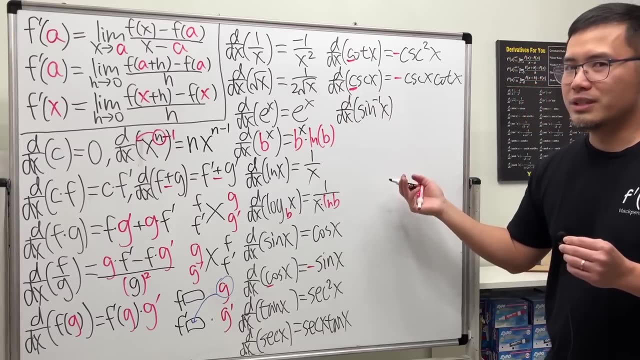 cos, sec x, and then its best friend is exactly that. so cot x. These are all the trick functions. Let's talk about the inverse of that. So taking the derivative of the infersine x, in fact, you just need to know three. 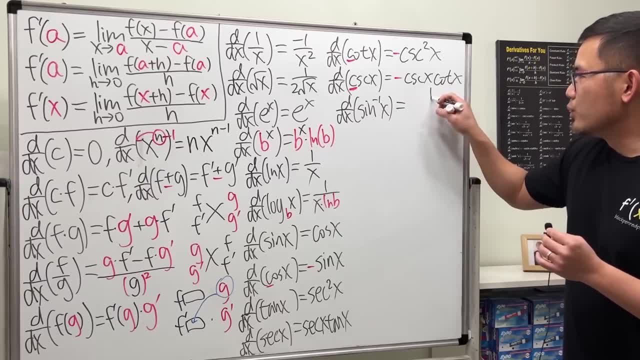 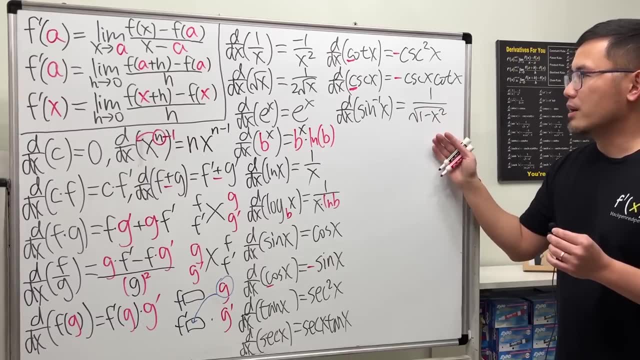 and the other three pretty much come for free. This right here gives you 1 over square root of 1 minus x squared. 1 goes first and then minus x squared. Why? Because the domain of infersine x is from negative 1 to 1.. 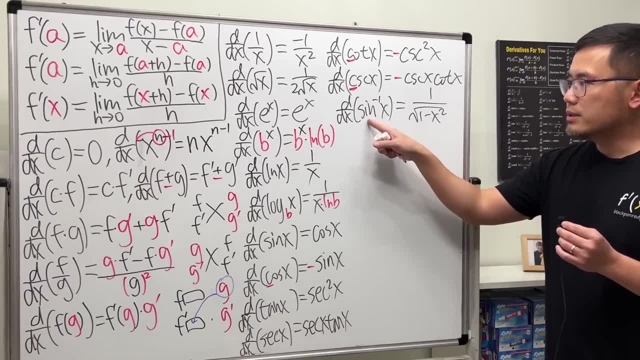 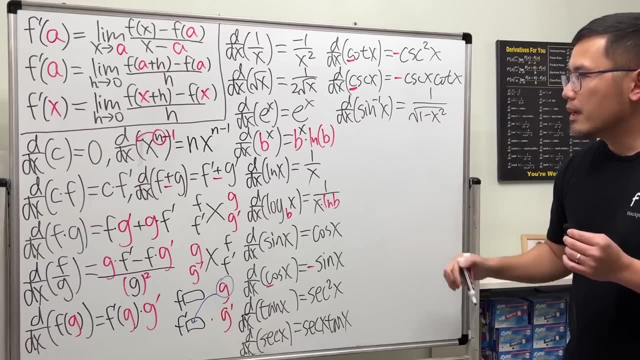 Likewise for this, But in fact the endpoints are not differentiable for the infersine function, so you also don't get the derivative if you plug in negative 1 and 1.. Once you know this, if you differentiate cos, sec, sorry. 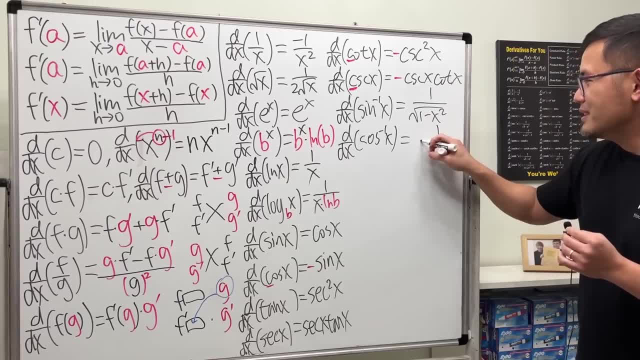 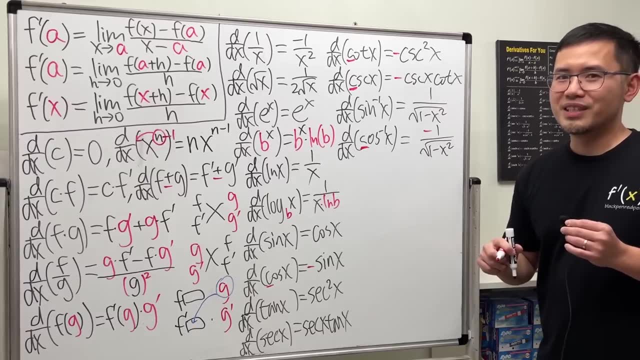 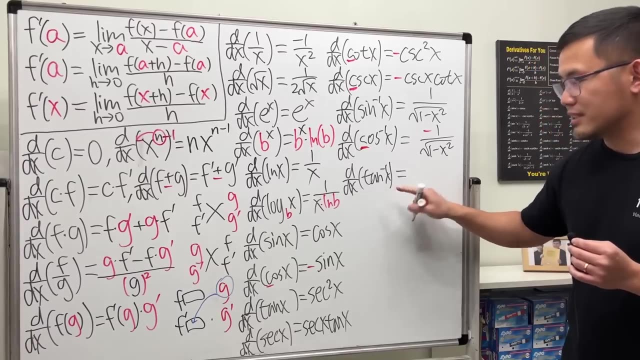 inverse cosine. it's just the same thing, but combining with what I told you guys earlier. we see the c. make sure you have negative derivative. Next one, let's talk about the derivative, The derivative of inverse tangent. you will see this a lot. 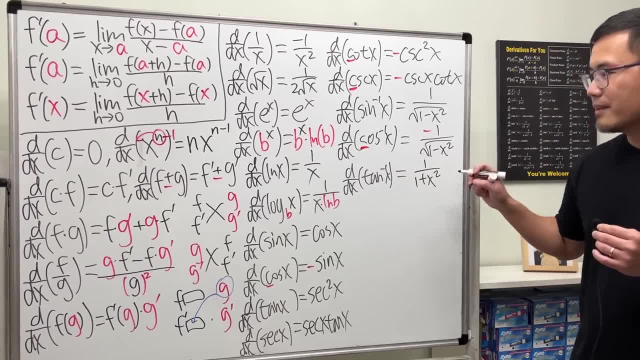 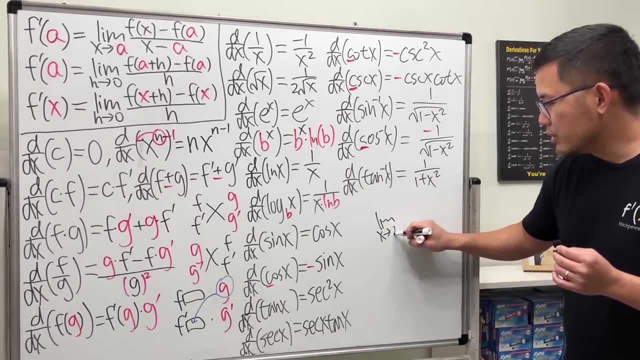 The derivative of this is 1 over 1 plus x squared. The domains for both of these are just all real numbers. By the way, the limit, as x approaches infinity, of inverse tangent of x is pi over 2.. You should also remember that. 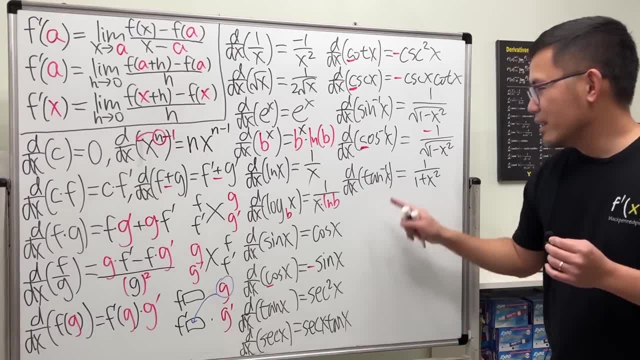 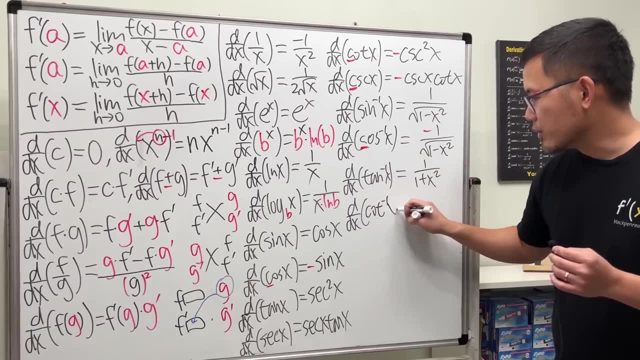 It happens quite a lot. Now, once you know this, you can expect to know the derivative of the co-function of that which is the inverse cotangent of x. Again, you end up with negative derivative and the same thing right here. 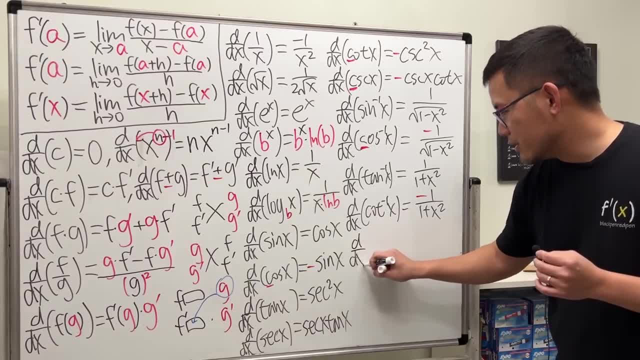 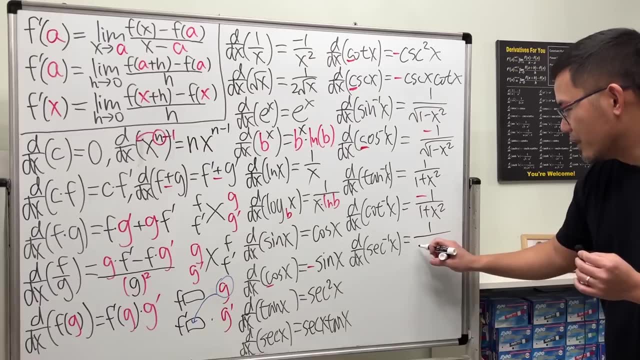 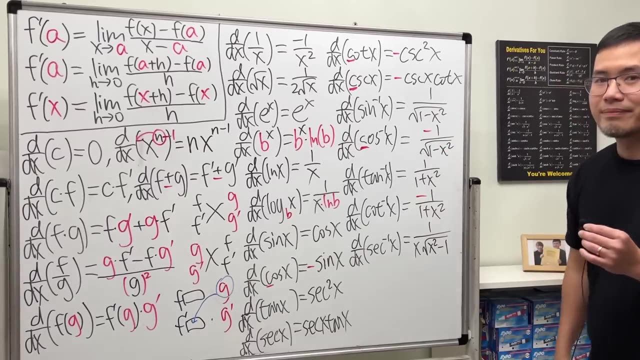 Now let's move to the derivative of inverse secant of x. Hopefully you don't see this one often right 1 over x times. the square root is the opposite of this: x squared goes first and then minus 1.. 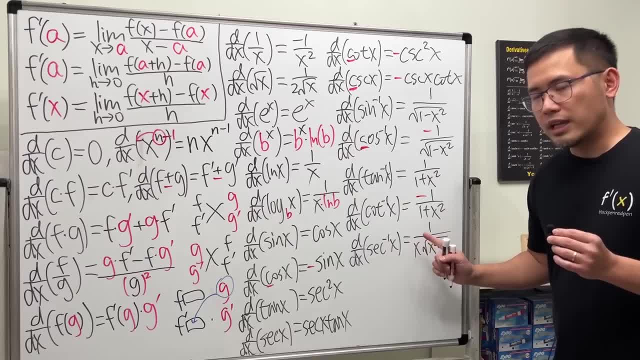 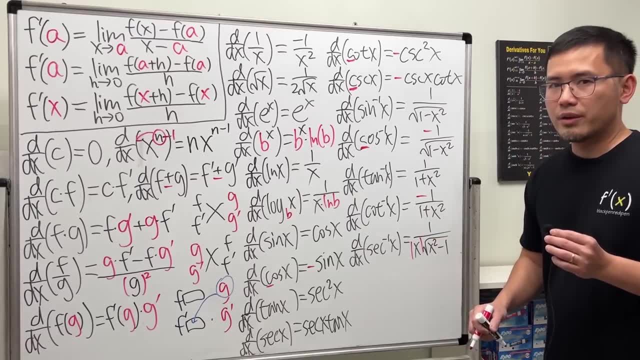 So here's the deal: If you use James Stewart textbook, then this is okay, but if you use other textbooks, then you will see an absolute value around the x right here. And the reason is depending on the domain, depending on how they. 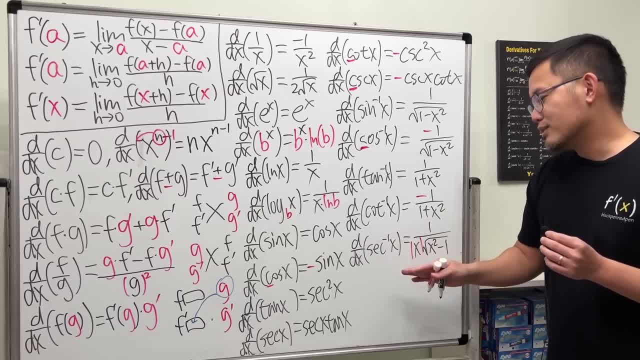 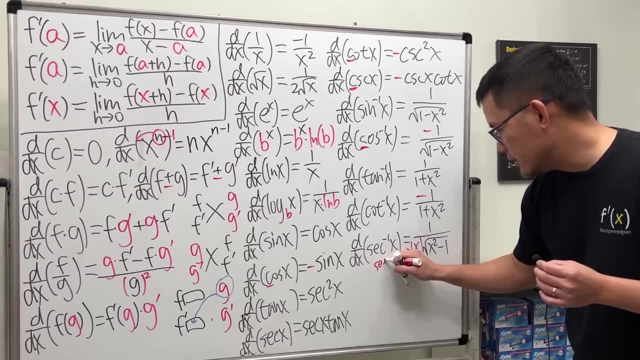 define the inverse secant. I don't really like this often, so I don't really ask my students this often. but I'll tell you this right here: depends on your textbook, So I'll say c textbook, And then of course you can also have